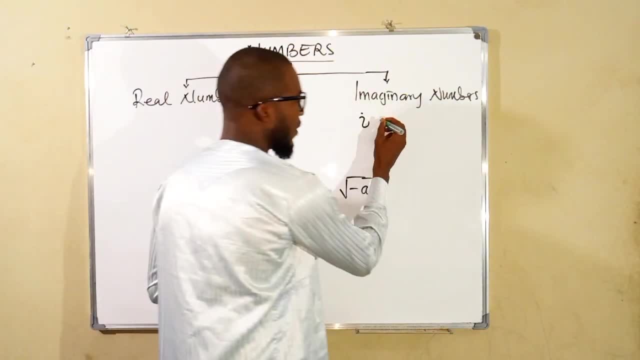 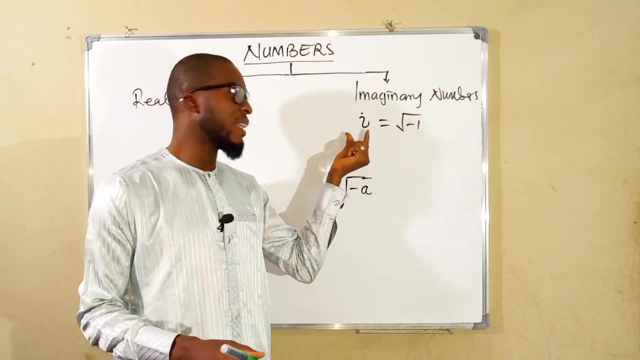 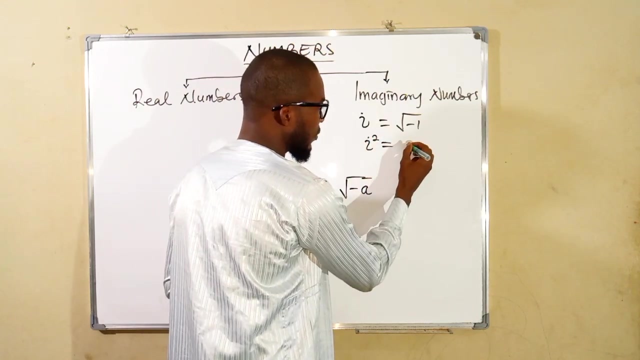 So imaginary number in mathematics is defined as the square root of negative 1.. If you take the square root of negative 1, you shall get an imaginary number, And if we square both sides we can have: i squared equals negative 1.. 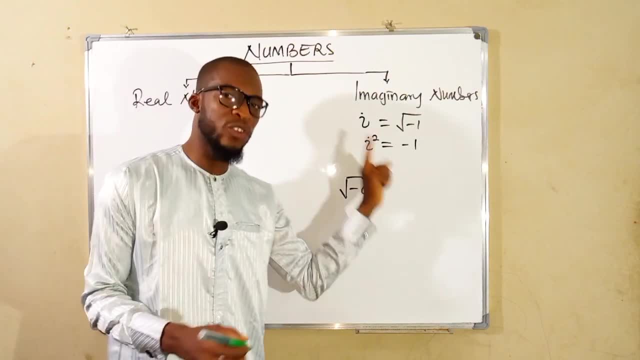 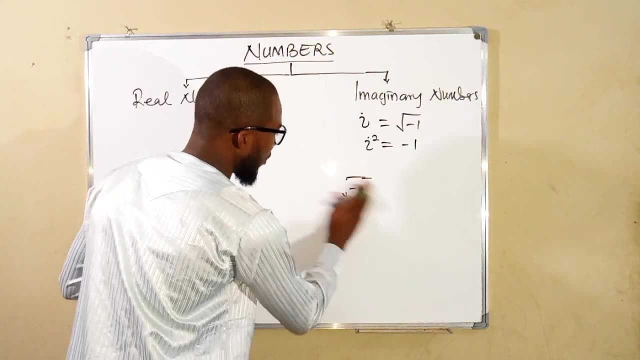 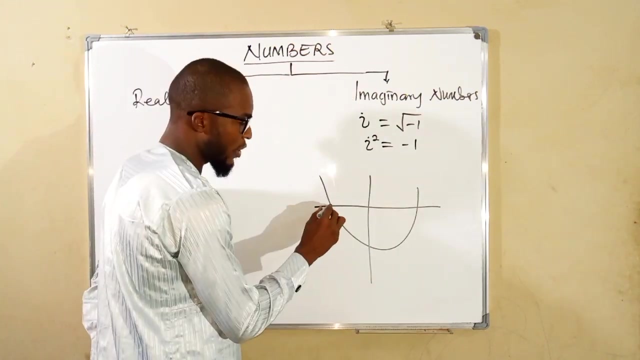 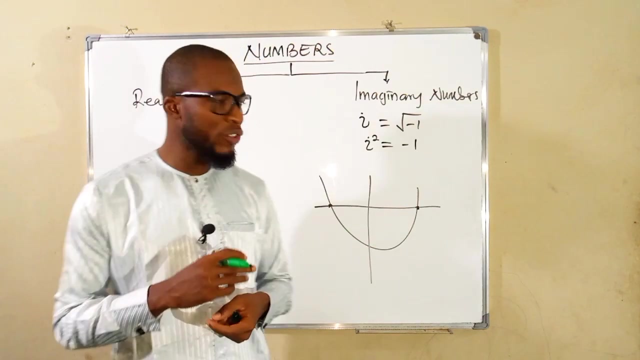 This means that if we square an imaginary number, we are going to obtain a real number. And another way you can remember imaginary numbers is in solving quadratic equations. You know if you have a quadratic graph in this form. So the two points where the parabola touches the x-axis are the real solutions of that quadratic equation. 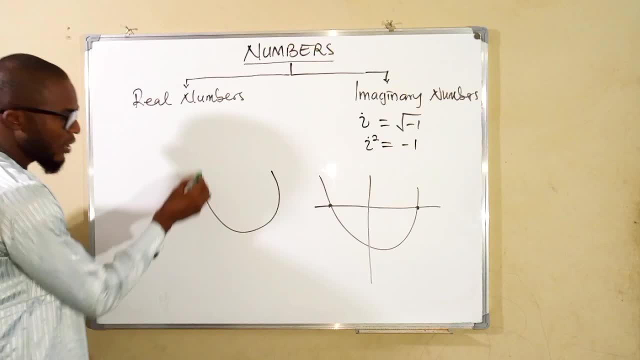 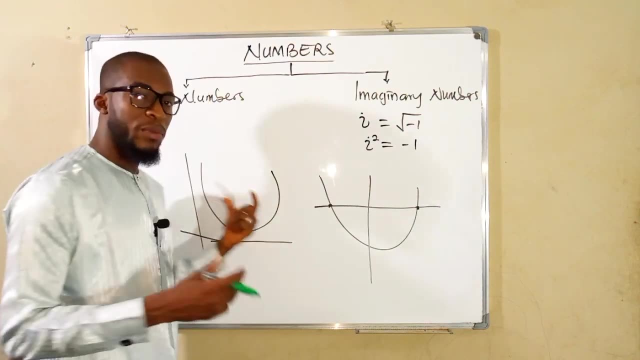 But sometimes we may have a quadratic equation that passes with a negative number Without touching the x-axis. So in that case we say the solution is imaginary Because the parabola didn't touch the x-axis. So this is another way. 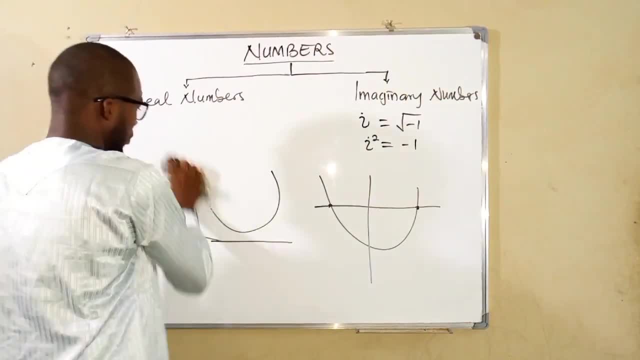 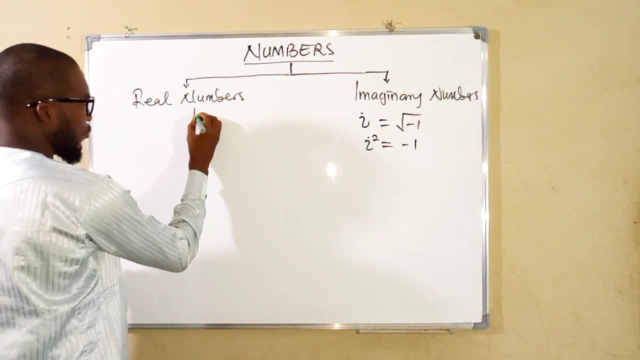 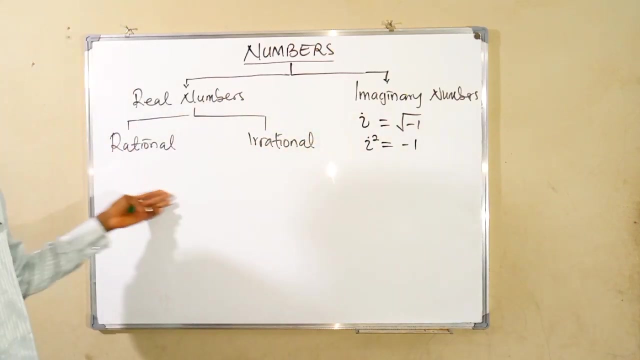 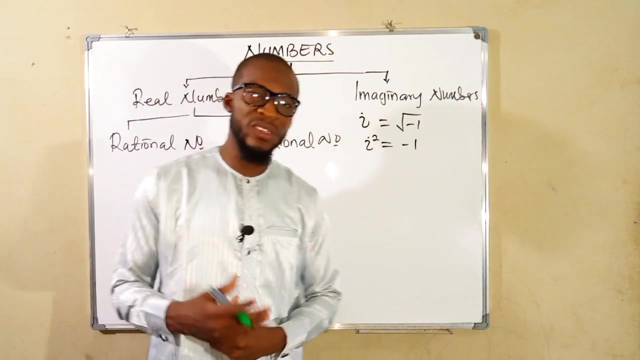 Coming back to real numbers, Real numbers are subdivided into two forms, again Two categories. We have the rational numbers And we have the irrational numbers. So what are rational numbers? Rational numbers are those numbers that can be expressed as a ratio of two integers. 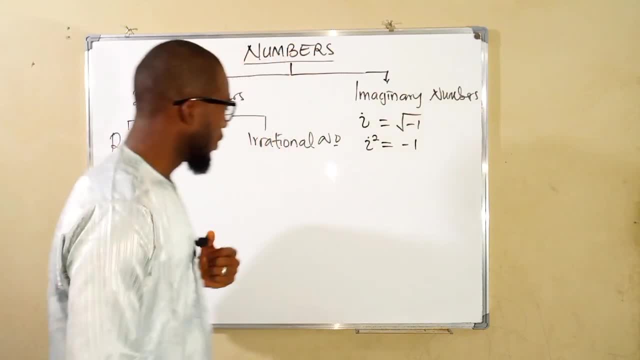 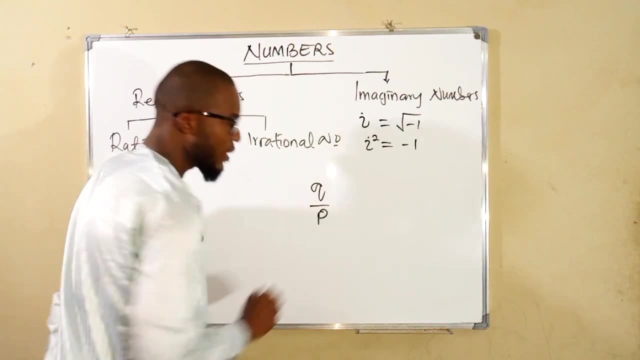 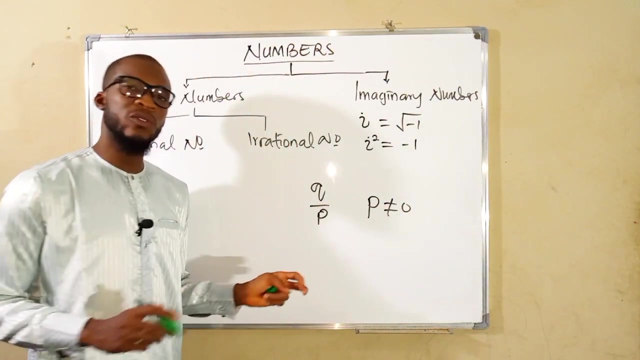 We are coming to integers. I will explain integers in details for you. Once a number can be expressed as q over p, Where p and q are all integers, But p is never equal to 0. Because to express two numbers in ratio. 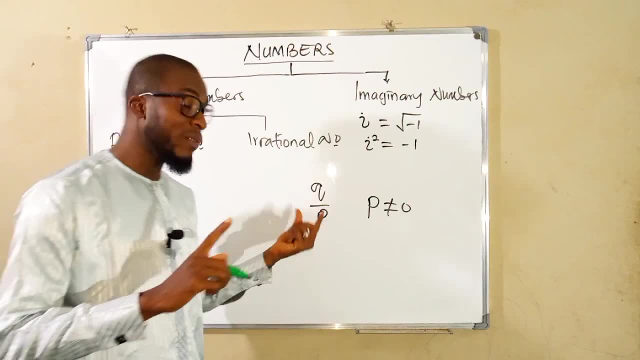 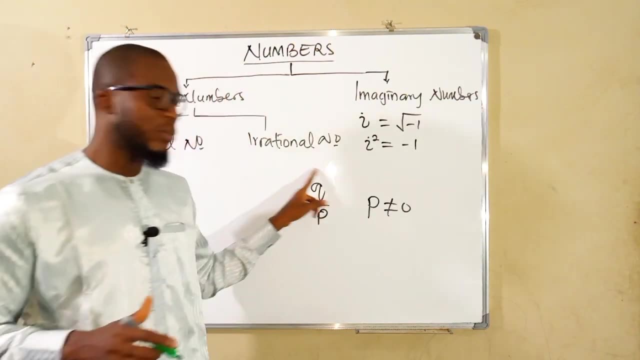 The denominator will never be equal to 0. Because if the denominator is equal to 0. We say that statement is undefined. So once a number can be expressed in this form, We say it is a rational number. Example of these rational numbers: 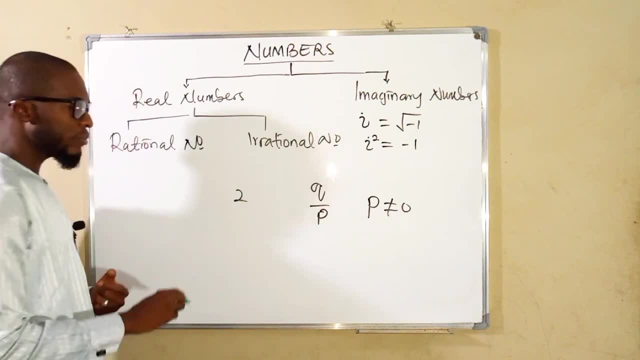 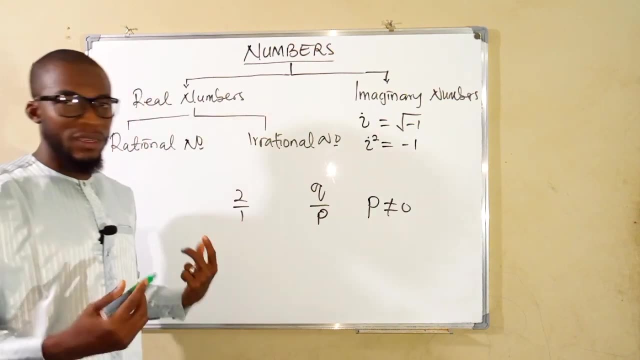 We have a whole number like 2.. Because 2 can be expressed as a Fraction. So we can say 2 over 1 is the same 10 as 2.. We can say 10 over 5 is the same 10 as 2.. 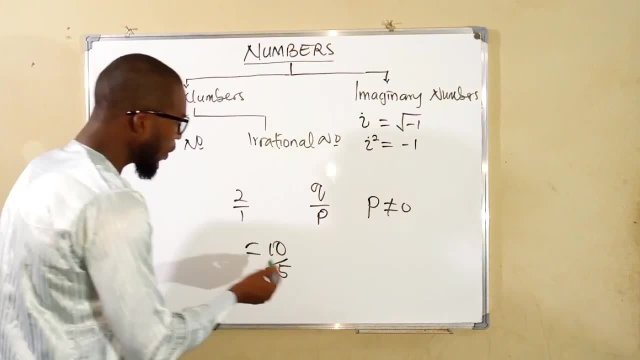 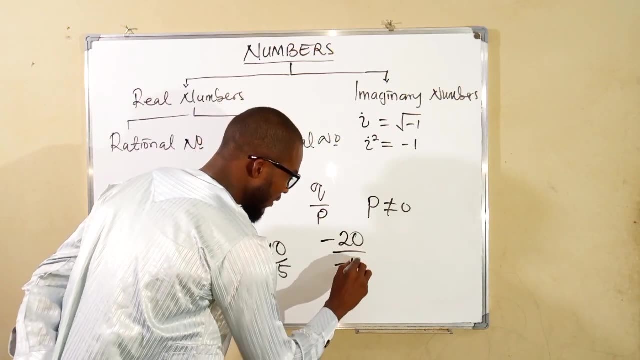 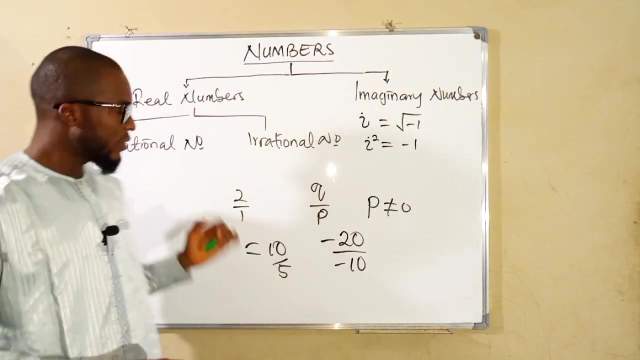 Because 10 divided by 5 is 2.. We can say negative 20 over negative 10 is the same 10 as 2.. Because negative cancel, negative 20 divided by 10 is 2.. So these integers, All integers, are rational numbers. 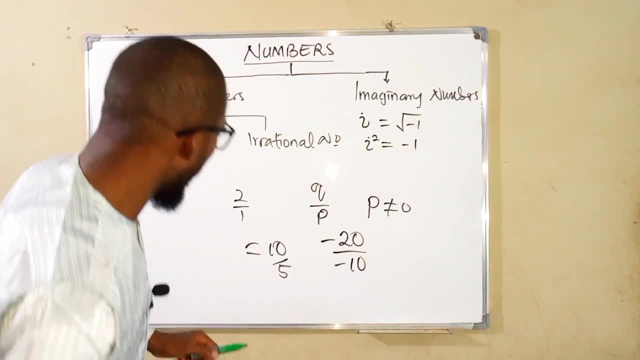 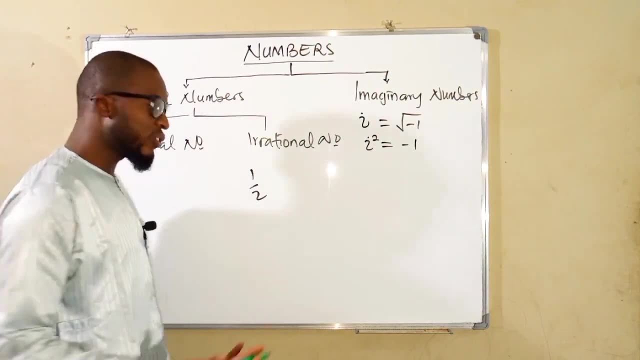 Another form of rational numbers. We may have ordinary fractions Like 1 over 2.. 1 over 2 is a fraction. It is also a rational Because it is expressed as ratio of 1 and 2.. 2 over 3.. 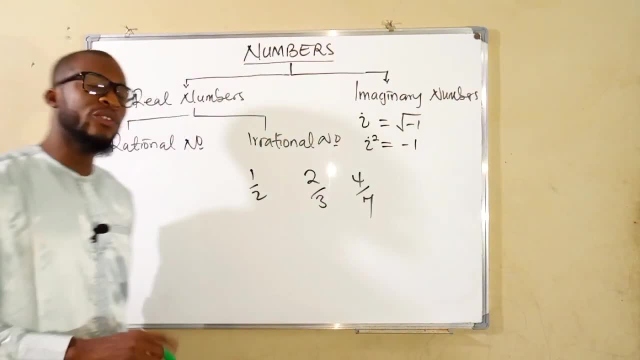 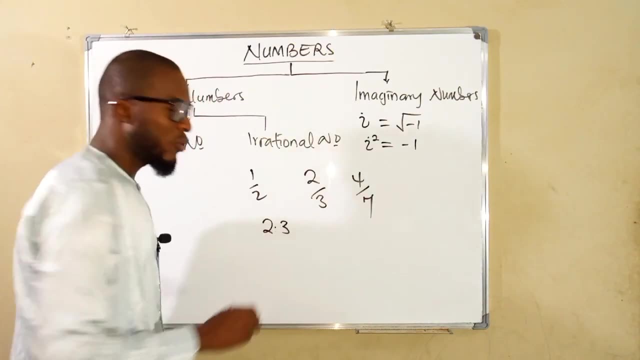 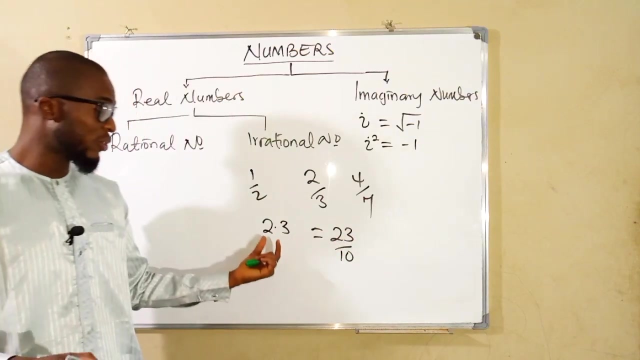 4 over 7.. They are all rational numbers. Another form of rational numbers. We have decimal numbers like 2.3.. 2.3 can also be expressed as 23 over 10.. You can see, because 23 divided by 10 will give us 2.3.. 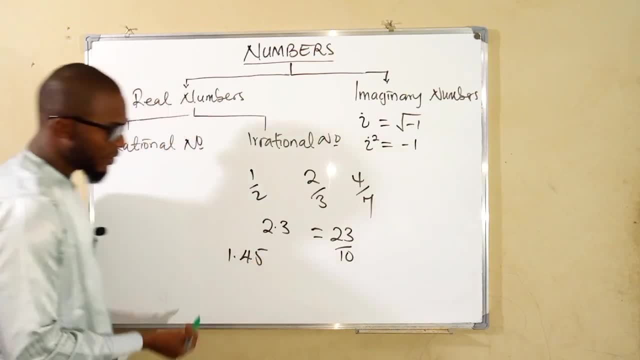 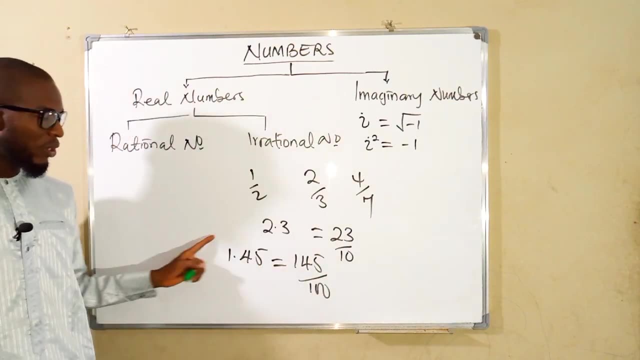 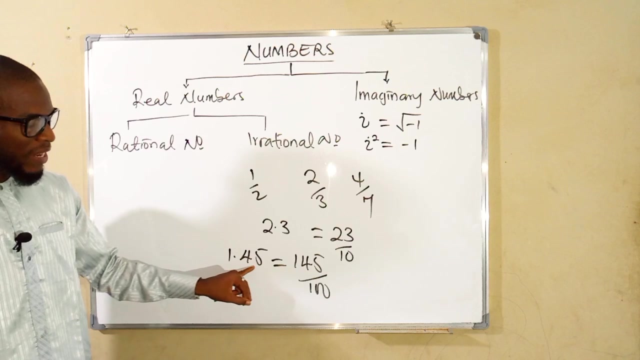 We can have 1.45.. This can be expressed as 145 over 100.. This is the same thing as this. Therefore, this decimal number can be expressed as a rational number. But look at it, We have a terminating decimal number. 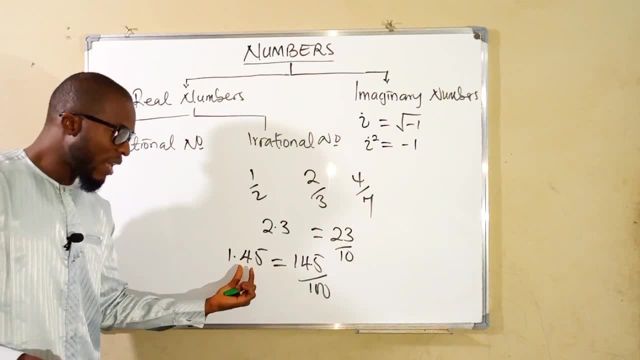 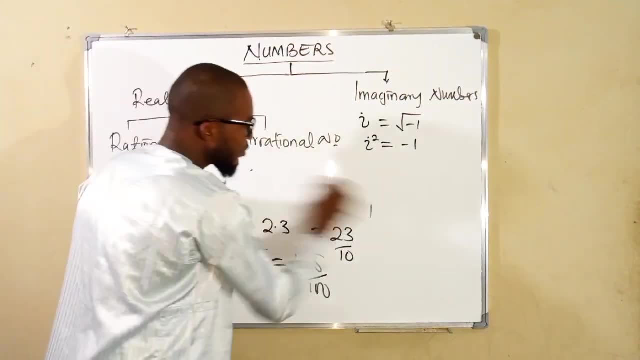 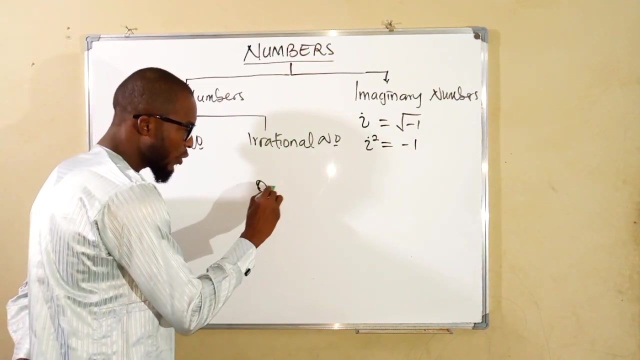 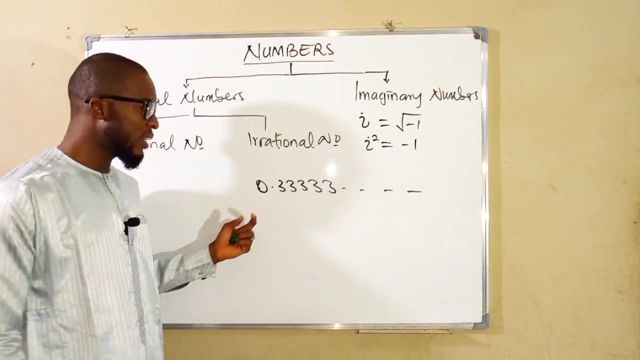 Terminating in the sense that it has an end. We have only two decimal places here. Sometimes we may have non-terminating decimal numbers Like 0.333333.. But they are recurring In the sense that 3 is repeating. 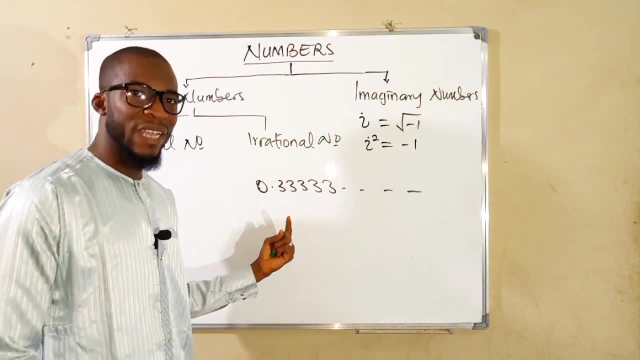 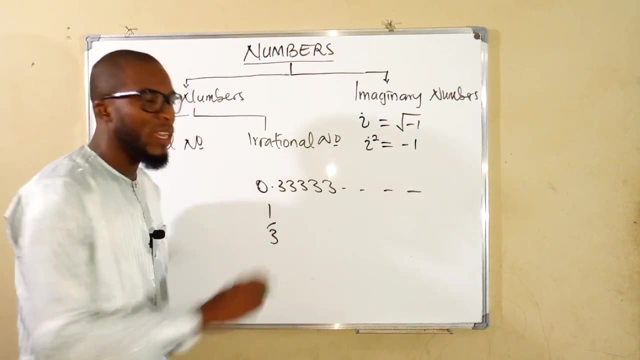 It keeps on repeating, But it is non-terminating. These types of numbers are also rational numbers, Because it can be expressed as 1 over 3.. In our next class, I am going to show you how to transform these decimal numbers into fraction or rational numbers. 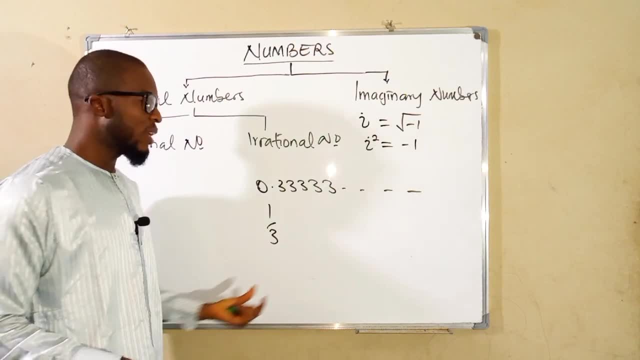 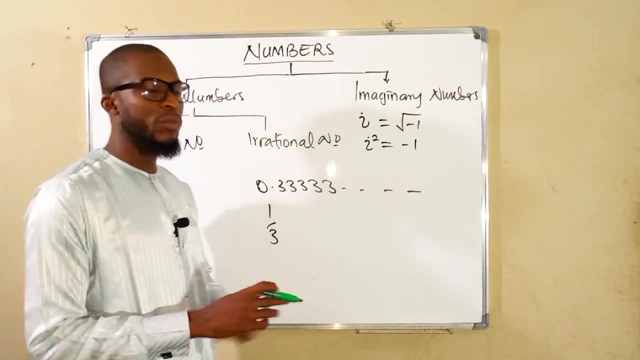 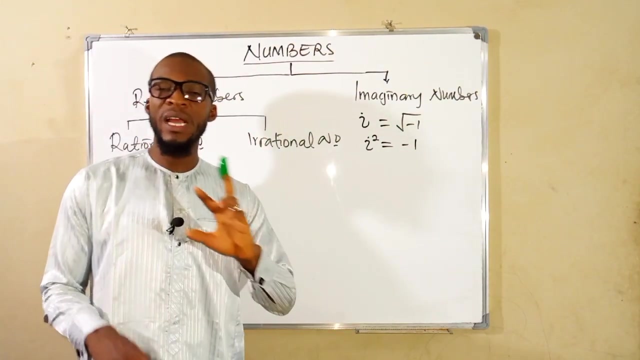 So terminating decimal numbers and the non-terminating decimal numbers, which recall values, We see they are all rational numbers. So, coming back to irrational numbers, Irrational numbers are numbers that cannot be expressed as a ratio of two integers. Example: 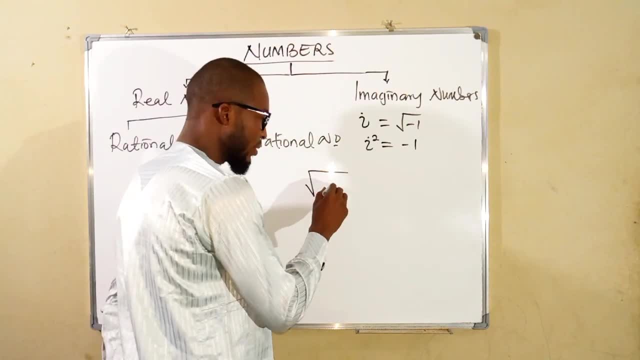 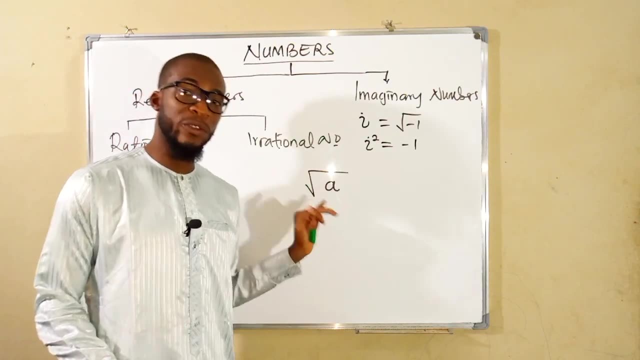 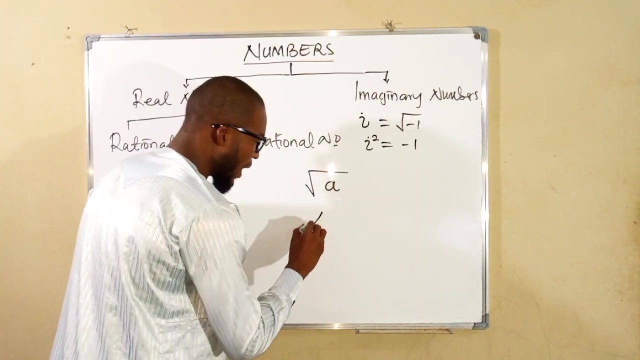 A square root of a rational number, Any rational number A square root of a rational number, If, and only if, that rational number is not a perfect square number. We see, it is irrational. We know pi. We say pi is an irrational number. 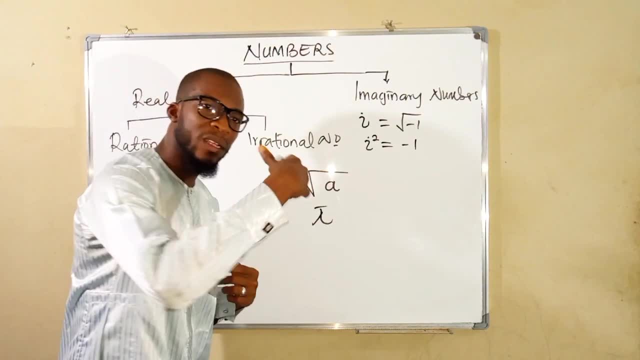 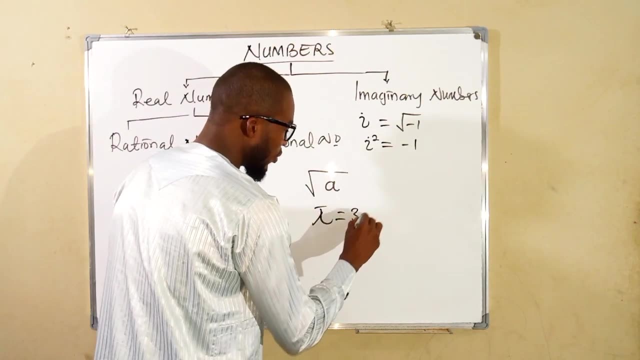 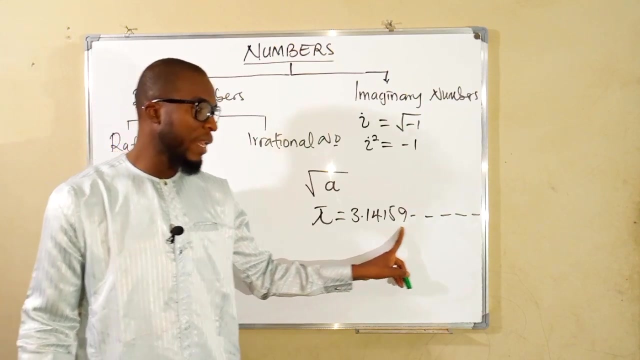 Because it has non-terminating decimal values that are not recorded, Which is approximately equal to 3.14159, and so on and so forth. You see these numbers, they are not repeating And they are non-terminating. So we see it is an irrational number. 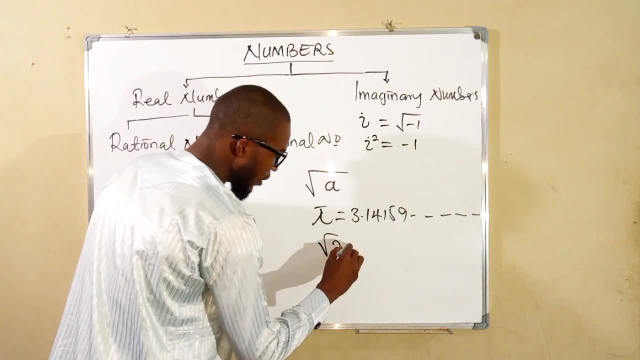 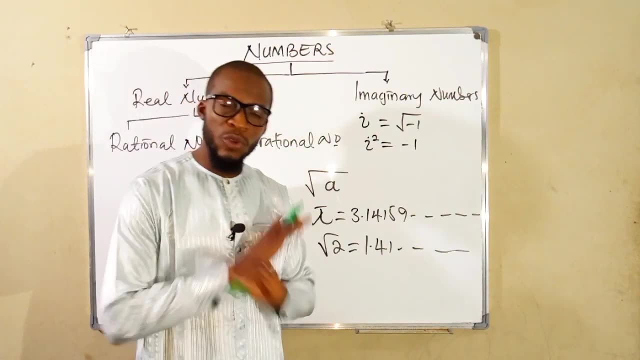 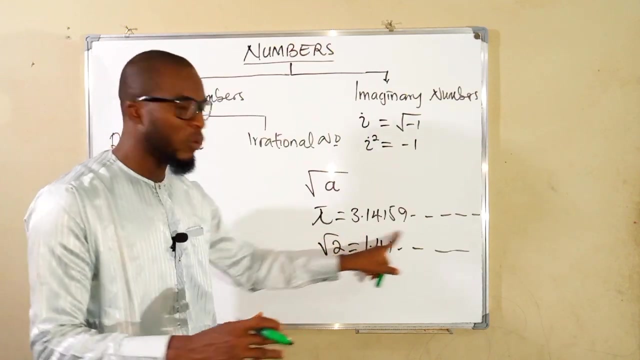 Square root of 2 is something like 1.41.. It keeps on going, Non-terminating, Non-recording, So it is an irrational number. We cannot find two values that can be expressed as a ratio of this. So, coming back to rational numbers, 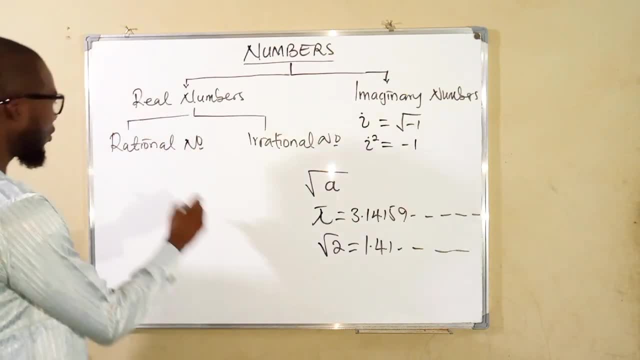 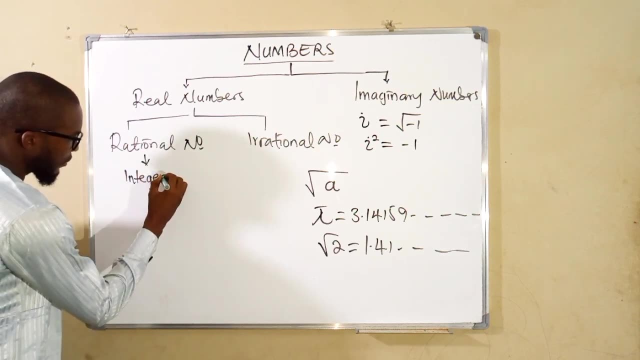 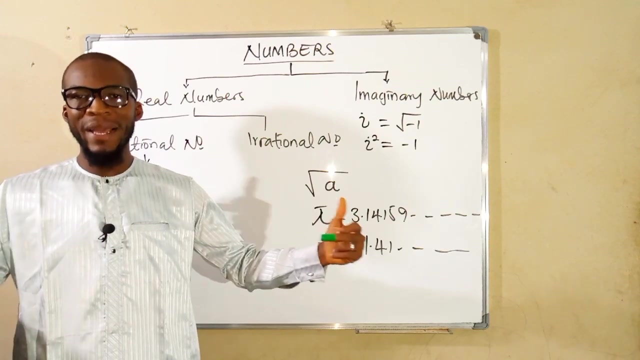 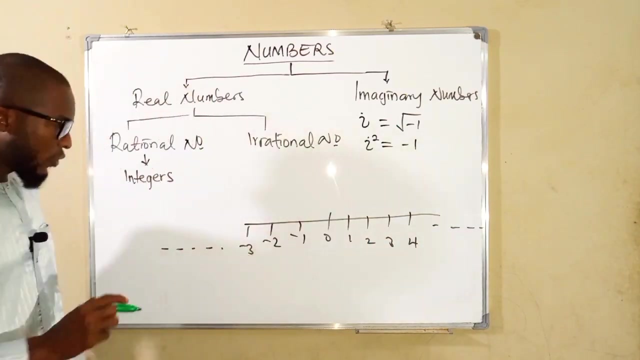 We have other subset of these rational numbers And the first one we have are the integers Integers. Integers are just those numbers on the number line. This is a number line. Every number you can see on a number line is an integer. 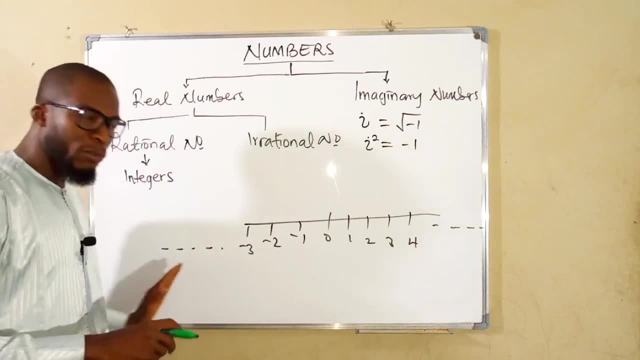 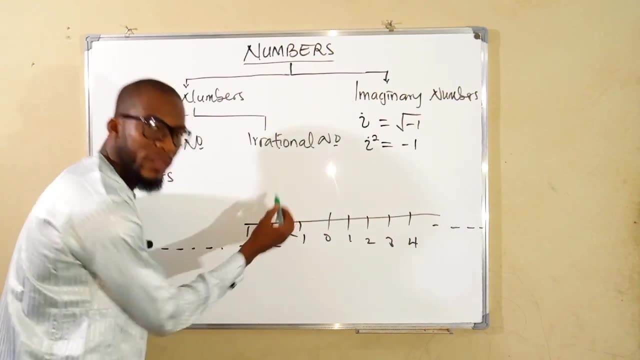 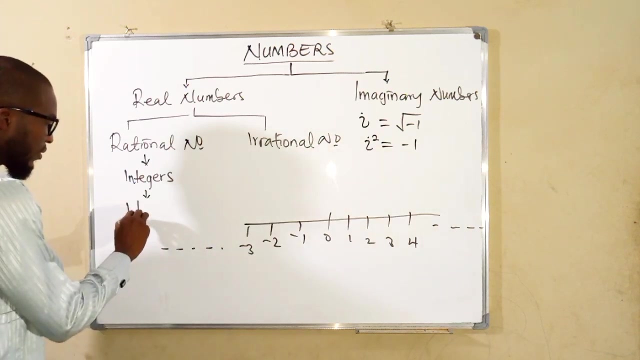 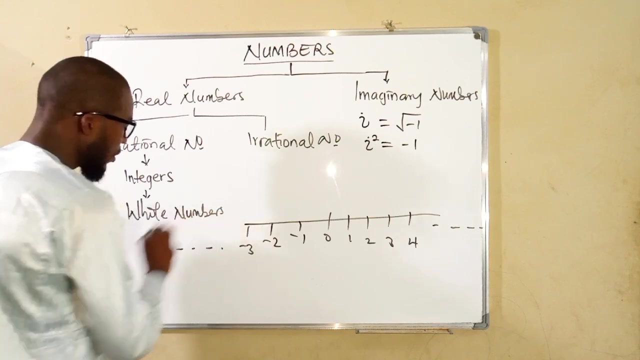 We have the positive numbers, We have the negative numbers Including zero. They are all integers Excluding the numbers, Excluding the numbers in between them. So under these integers, we have whole numbers. We have whole numbers. Whole numbers are a subset of integers. 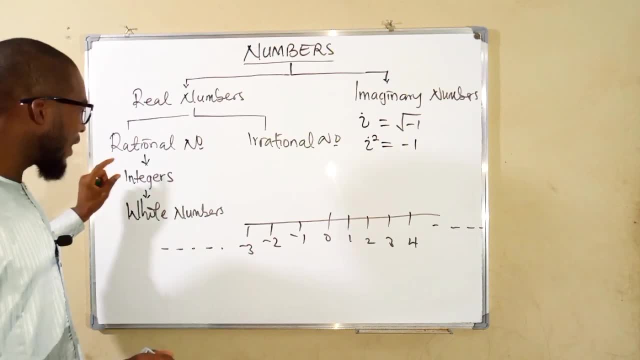 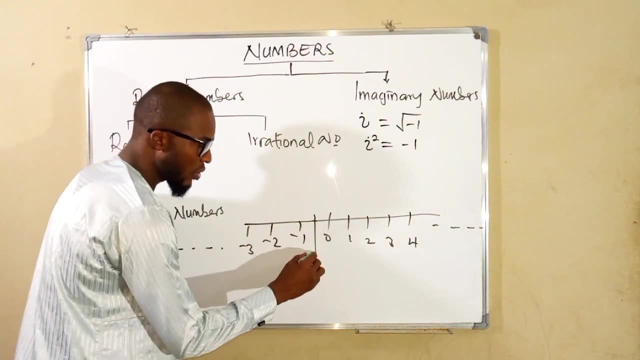 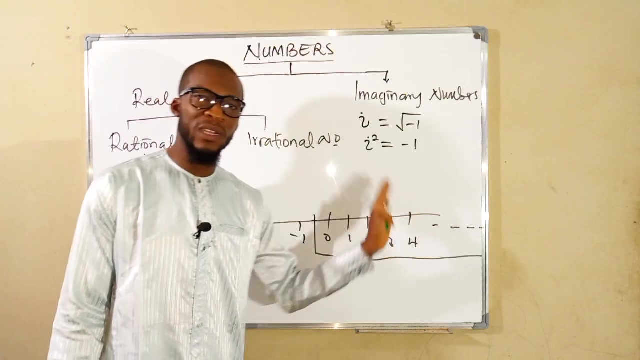 Because all whole numbers are integers, But not all integers are whole numbers. Alright, So whole numbers begin with zero And any other number to the right. So we have zero, One, Two, Three, Four, Five, In that order.